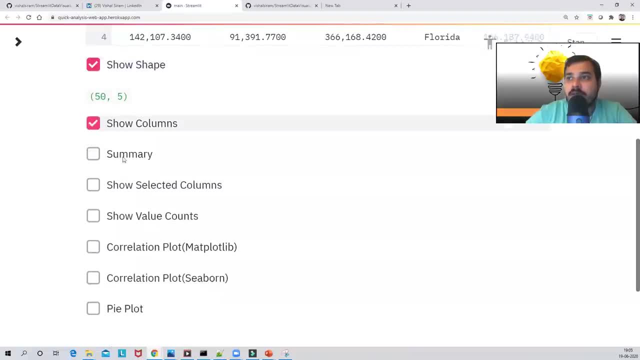 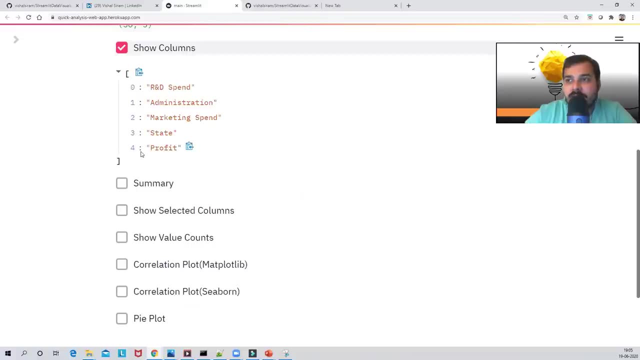 shape. If you click on this, you'll be getting this information. show columns. You can see that you are getting this all particular information. Now, this is amazing because this is doing with the help of Streamlit library itself. You want to see the summary? 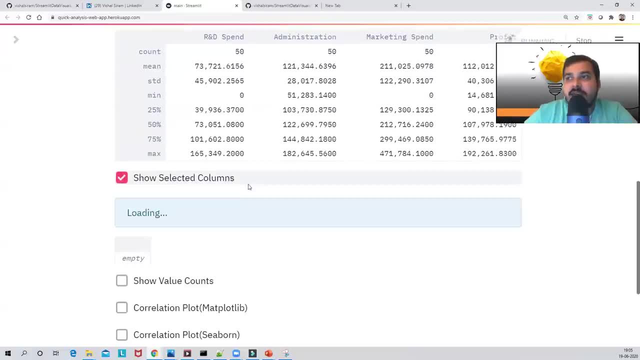 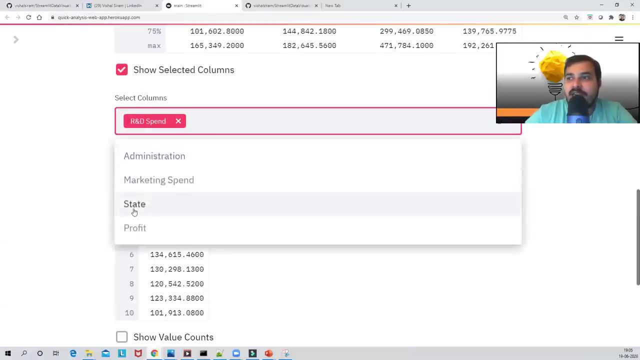 just by one click you're able to see this information. show selected columns. Suppose you want to select any specific column as like R and D spend. So this is the value that you are actually getting If you want to select some states column. so you are getting in. 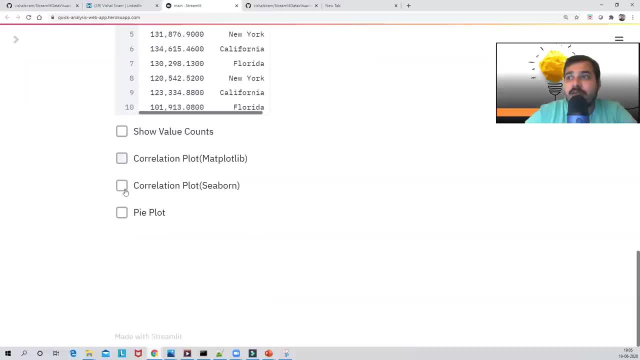 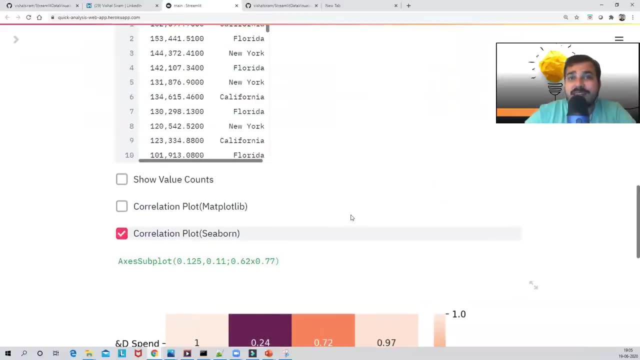 this particular way you. he has also added, with respect to the correlation plot in Seaborn, How wonderful the diagrams will get displayed. This is the correlation. Yes, it is not pretty much advanced by guys, but he has at least started this, which is pretty much important. 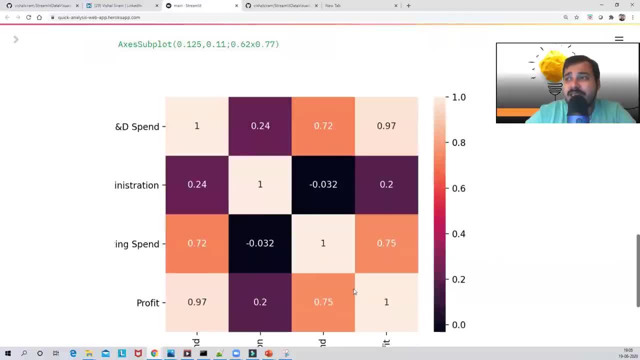 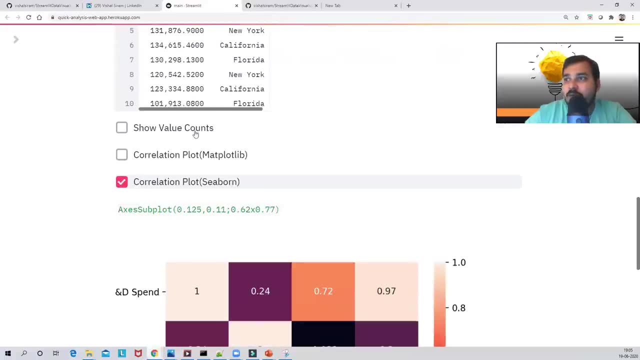 for the learning purpose. Now, still, we can add many more functionalities. We can see how many missing values are there. We can see how many unique values are there. I think he has done with respect to the unique values also. Okay, let's see: show value counts. 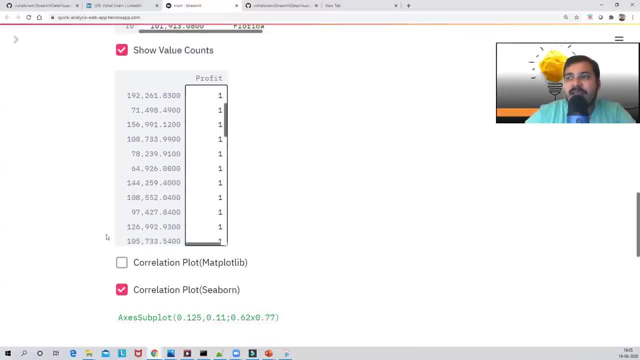 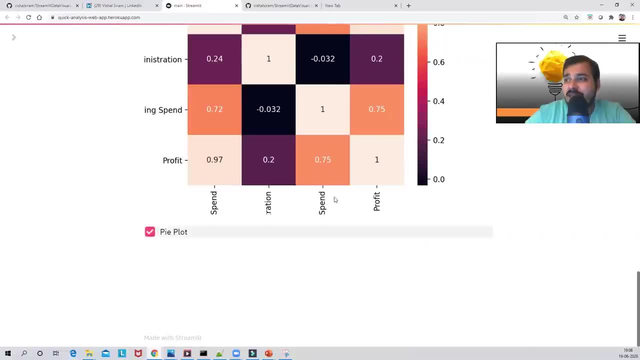 So he's given this. I think this he can actually make it more, look more better with more functionalities, But yes, it's a little bit more complicated, but it's a little bit more complicated, So it's a good start. He has also done pi pi plot, but I think pi pi plot does not display. 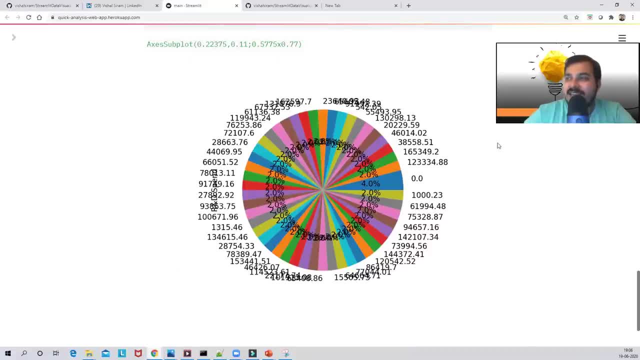 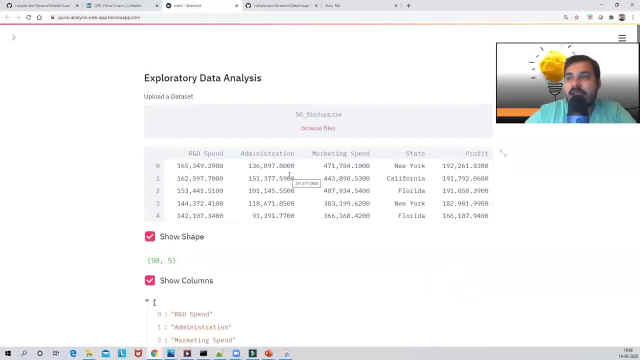 the data properly. So this is how it gets displayed. Again, this needs to be improved, Definitely. You can definitely add a lot of functionalities apart from this, but you can see that how light weight it is actually One more issue that I faced in this particular. 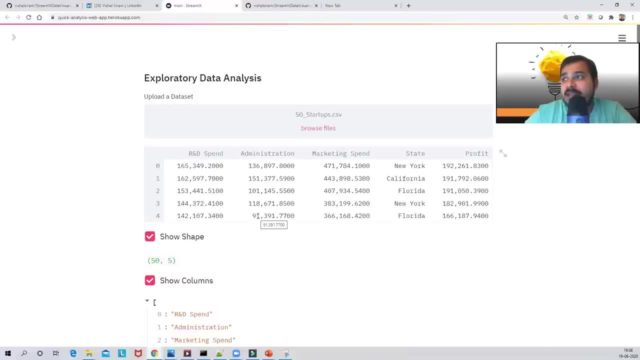 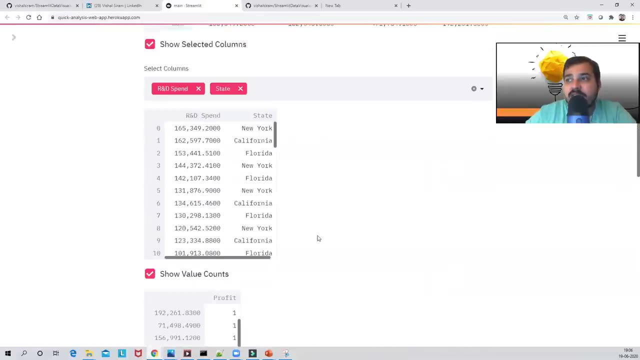 application is that if I'm trying to upload a huge data set, at that time this works a little bit slow and obviously it will be working. but we can make it better. So definitely try to add more functionalities over time. So let's go ahead and add some more functionalities over here. The code is very, very much simple. 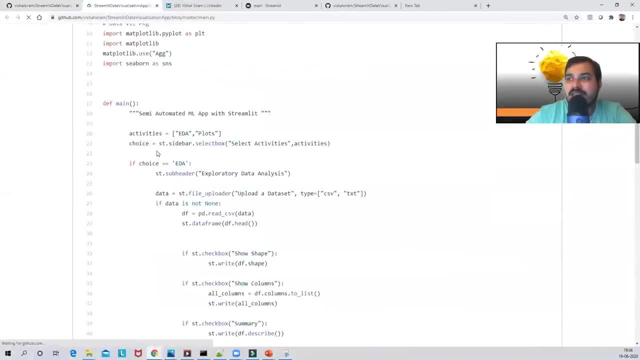 that if you just see the code for each and every functionality, suppose if I go and click on PDA EDA- sorry, here are the exploratory data analysis- He's just doing some kind of functionalities where he's reading the data set. He's displaying it right. So, with respect, 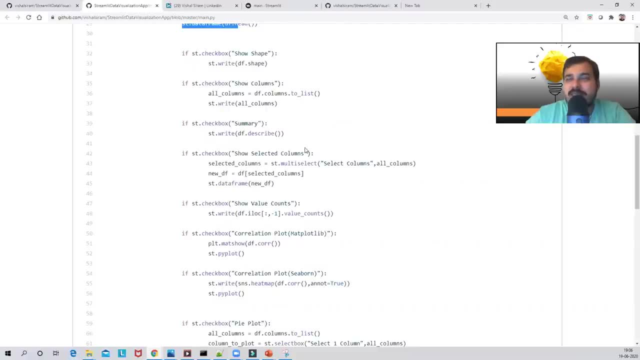 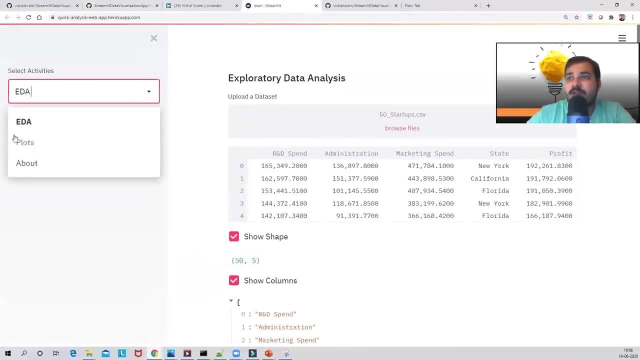 to each and every option is doing some Pandas operation. That's it. Pretty much simple code, but a very good start itself. Okay, So this is what the information. let me just go and see the next option over here with respect to the plots. 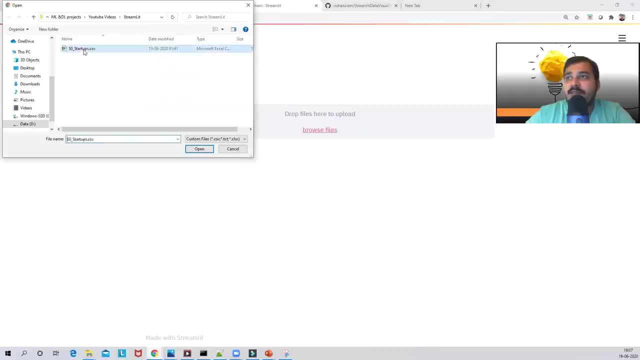 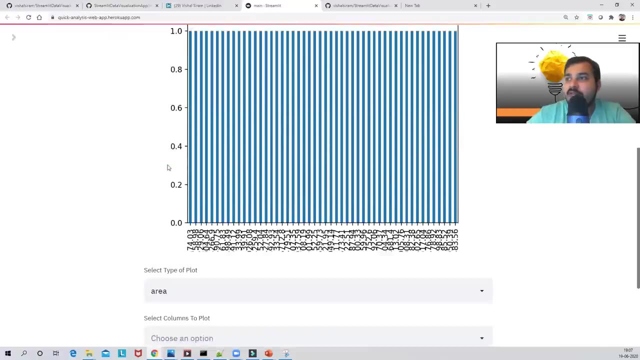 Okay, With respect to the plots, you can see I'm going to click the same file. Okay, So it will be uploading this whole file. Okay, Done. Show value counts. This is some data that is getting displayed. Now, suppose let me just select some area. Suppose I'm selecting. 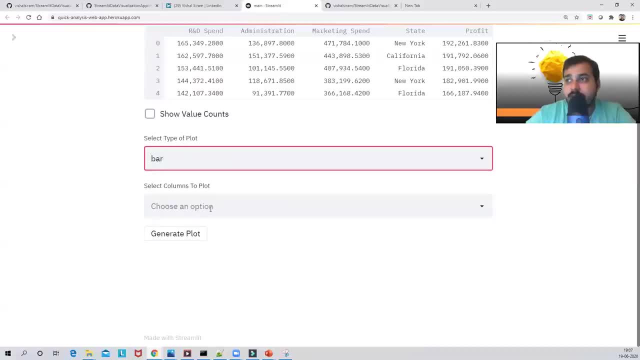 a type of chart plotting chart. Suppose I select bar And after that I select an option. Okay, I want to see the bar chart with respect to my R and D spent. And if I want to generate the plot, let's see. 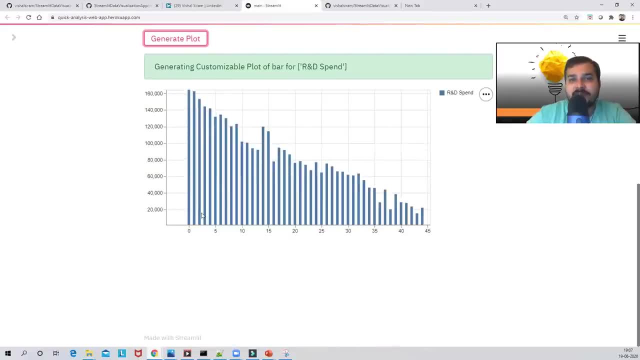 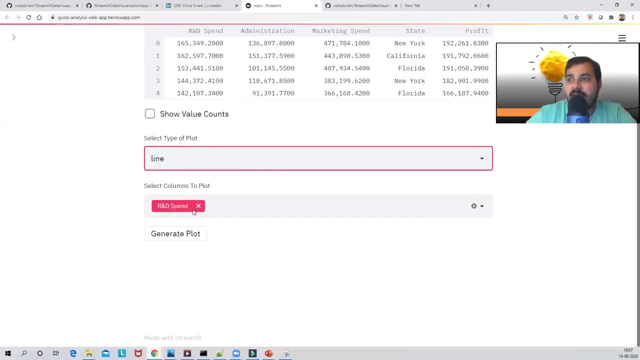 Quickly. you can see that how creatively it has actually created this particular graph- Right Amazing. Now the next thing is that suppose I want to try with line chart. Okay, I can also select multiple options, which looks pretty much amazing. Now this is how. 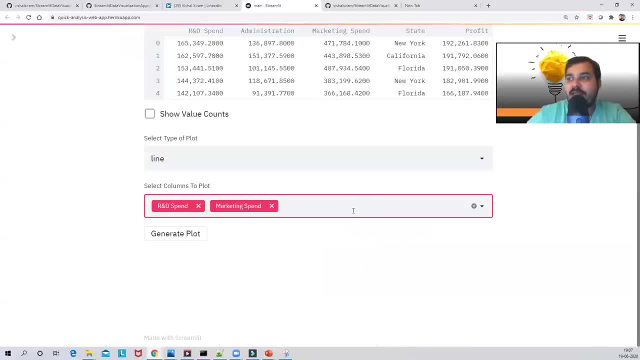 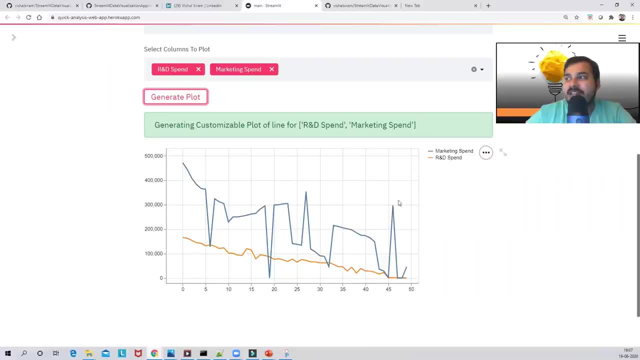 my line chart looks, Suppose I want to add some more thing, like market spend probably, And if I select the generate plot, you can see that you can easily compare the market spend and R and D spend. Okay, Market spend is varying a lot, but obviously by seeing 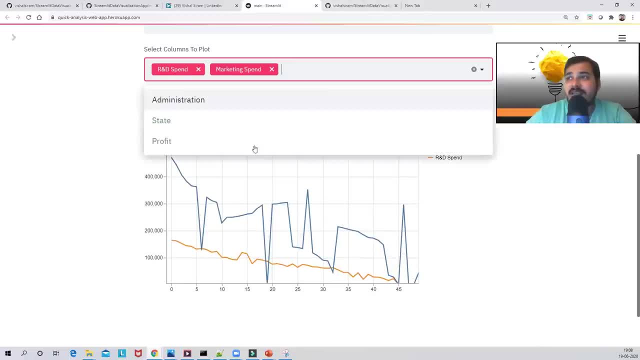 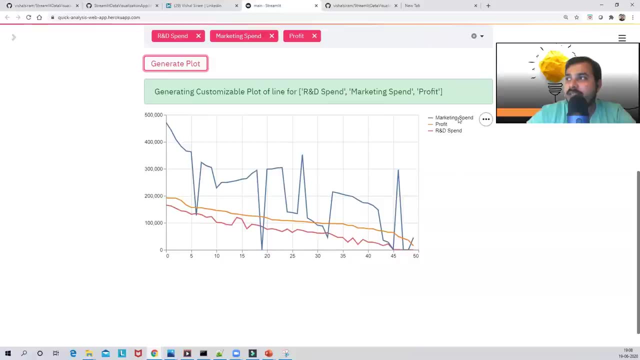 this: the marketing spend is more And if you are running a company, guys, usually market spend is more. Now let's see the profit, And if I generate the plot with respect to this particular profit, you can see that clearly how the diagrams are And you can save this. 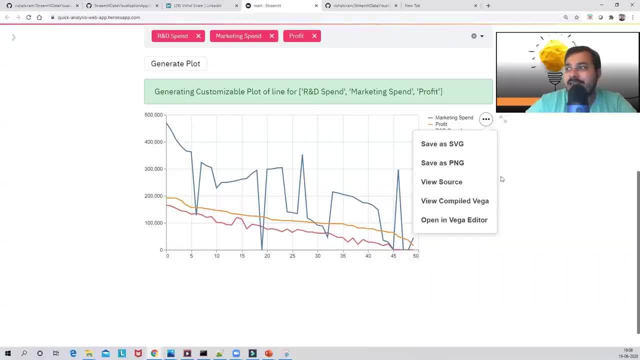 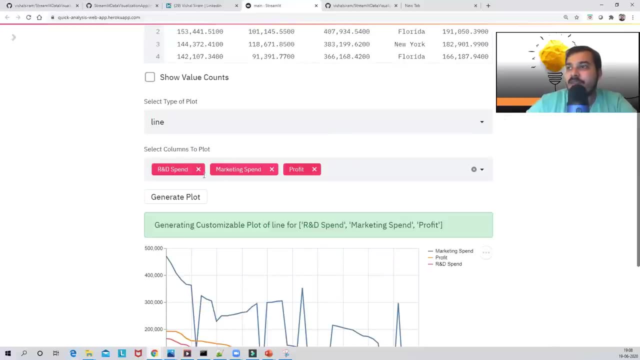 as an image PNG open in Vega editor. A lot of options are there right. So here you can see another very good image. If you right click also, you can also save this. Okay Now suppose if I want to compare with marketing spend and profit. So definitely see it brings. 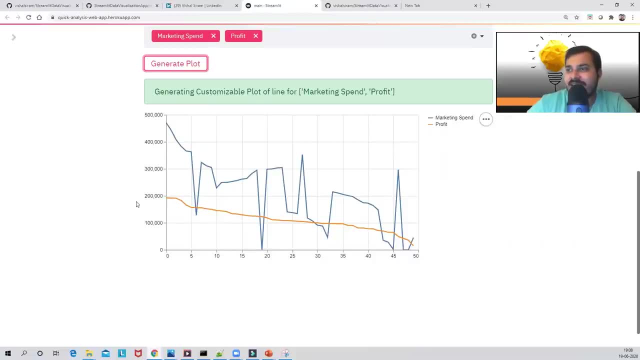 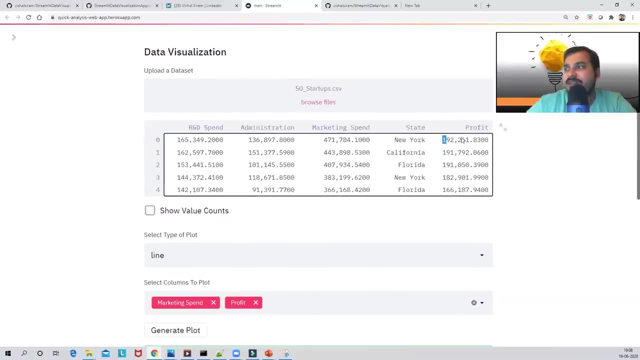 me to the market spend, So I can save this as an image. And if I want to compare with marketing spend, I can save this as an image. And if I want to compare with marketing spend, I can save this as an image. So, definitely see, this is the same thing. So this is what. 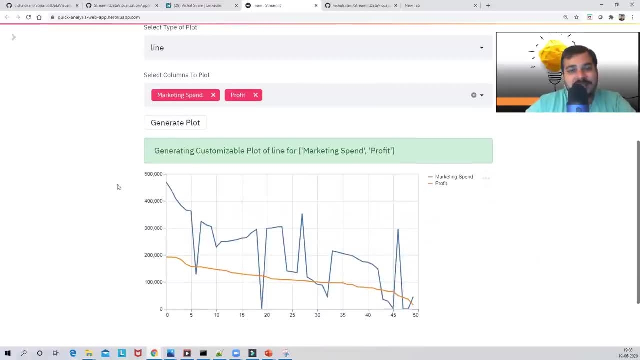 I see. So I can see that the profit is very, very less based on the market. The profit is very, very less. So what I see over here, but again, these units are at least different. but this is actually very upholders. Now, it is not a perfect image, It is just a very 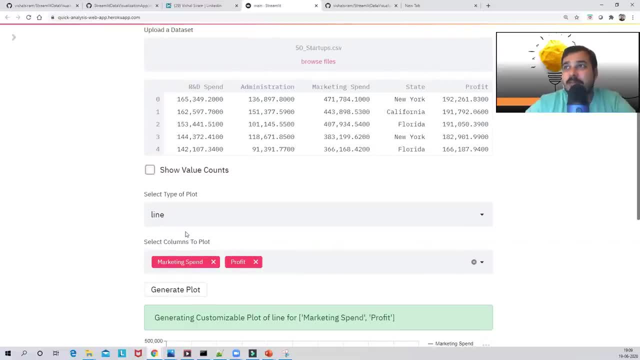 bad image, but basically they are the same, And one of the things that I really love about this is that these are the kind of images that you can have on your device. These are the kind of images that you can have on your phone, So this is very well known, It seems. 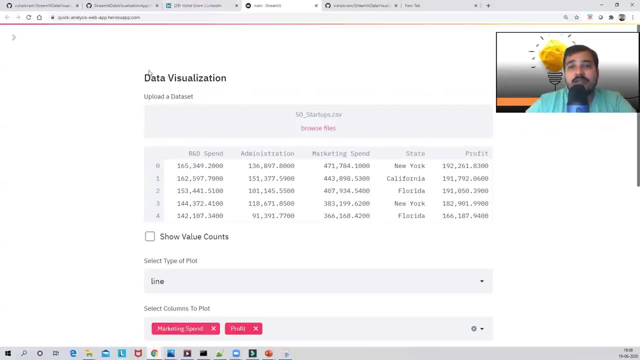 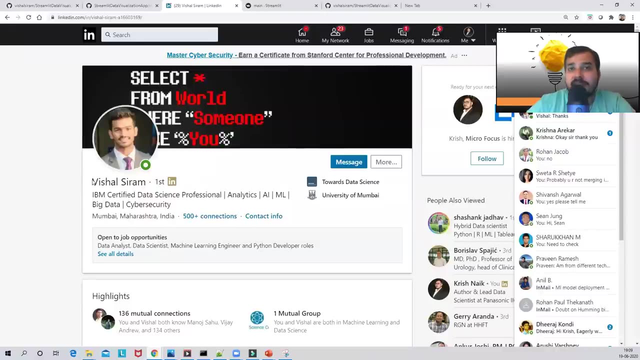 to me like I have the same image. So the last thing I want to talk about is that right now I don't really want to go too far into it because there's so many other things I want to talk about, But but I want to point out just one thing and I want to just kind of 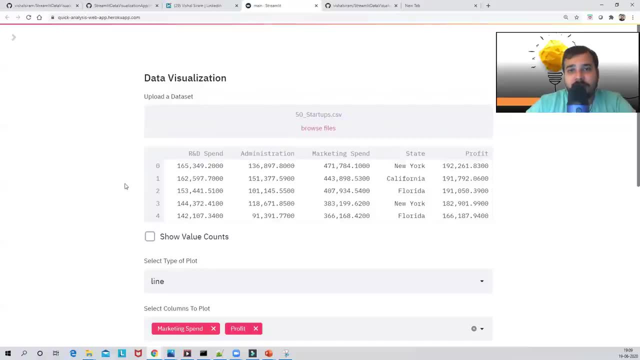 talk about this, So I want to talk about this today. guys, this was all about this particular video. i hope you like it. please do subscribe the channel if you have not already subscribed. i'll see you in the next video. have a great day, thank you, bye.